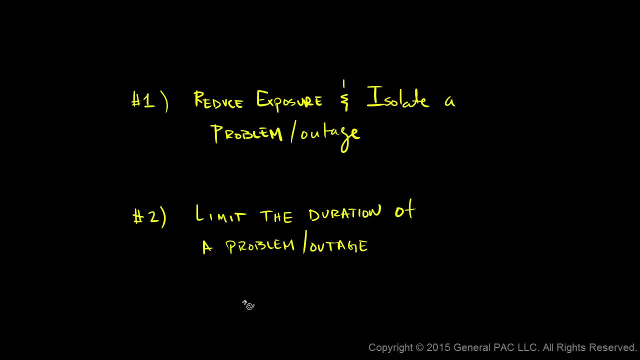 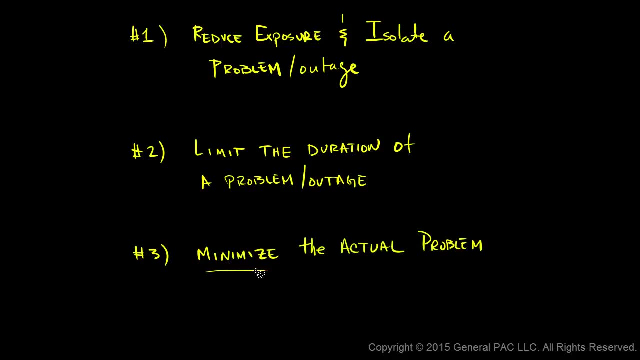 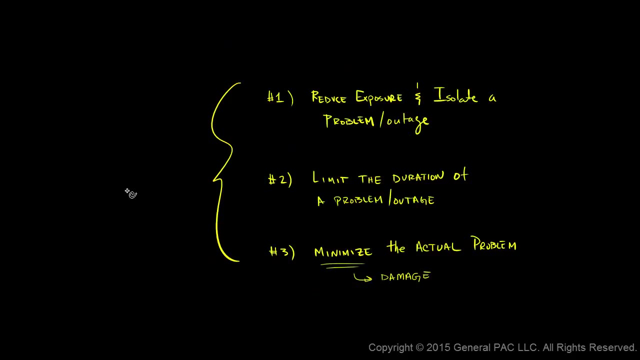 We don't want to take an outage longer than we have to. And 3. We want to minimize the actual problem, And what I mean by that is to actually minimize equipment damage. This is what we want from our electrical system, And coordination is going to help us achieve it. 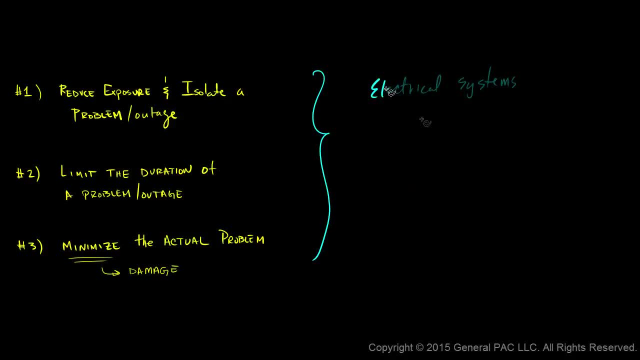 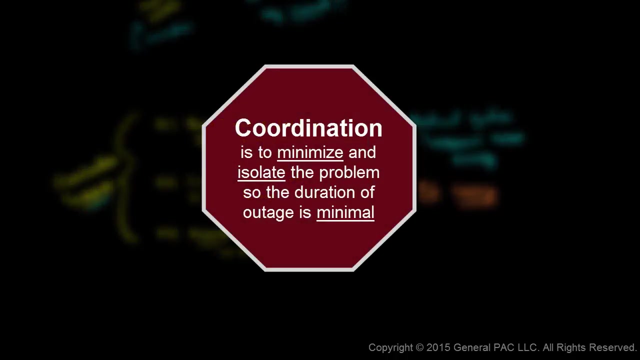 It's really important to keep in mind that electrical systems must be designed to prevent human injury, So the number one priority should be safety. So if we were to summarize coordination in a few and simple words, it would be: Coordination is essentially to minimize and isolate the problem. 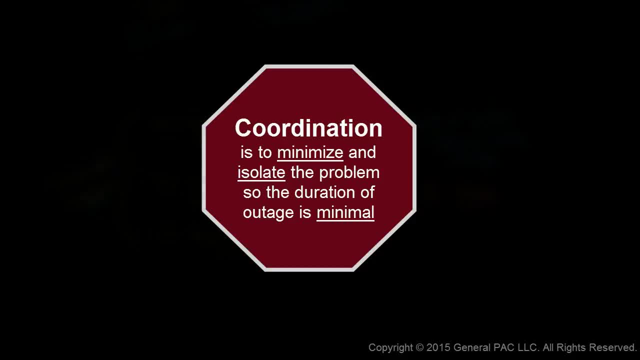 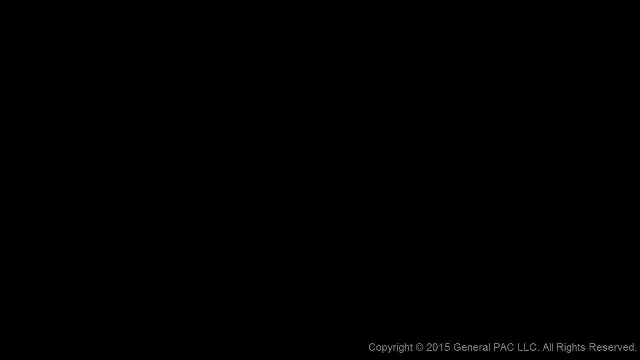 so the duration of an outage is minimal. So let's quickly give an example of this. So suppose that we worked at an industrial facility. So in this facility we might have a generator that's generating voltage, We might have an incoming line from a utility or the grid. 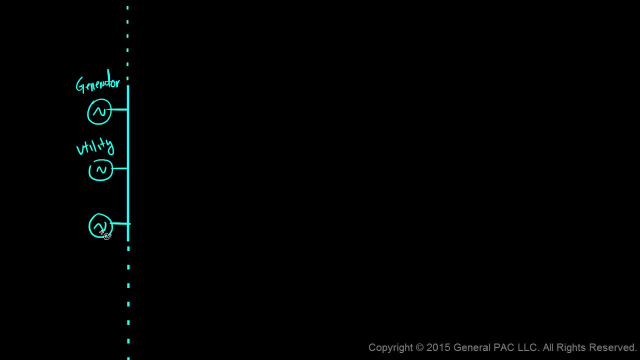 Or we may have some external source. Doesn't matter what, it is right As long as we're receiving power. And suppose that we have a breaker on the high side of a step-down transformer. So suppose that the generator was generating voltage at 12.4 kV. 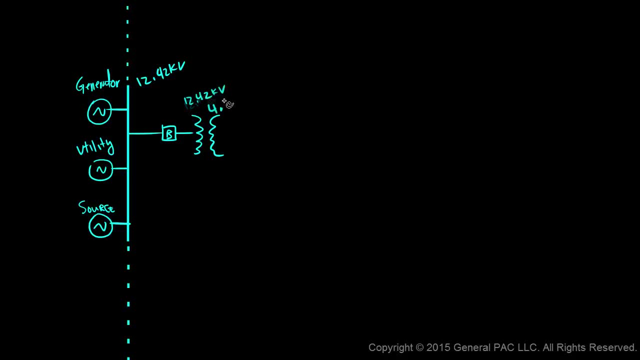 And the step-down transformer sets it down to 4.16 kV. And then it goes to the 4.16 kV bus And on that bus, let's say, we have a tap And this tap is fused and it's going to a motor. 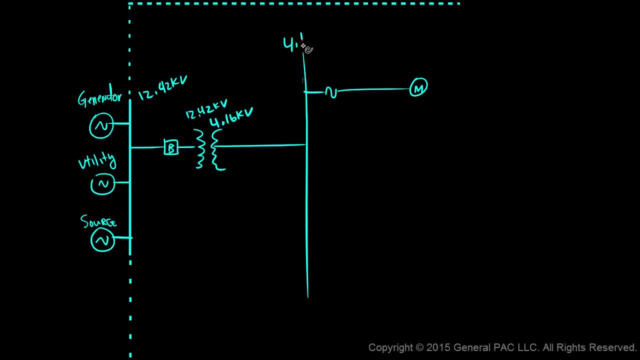 And this bus here is 4.16 kV, And then we have another tap and another motor. So keep in mind that this right here is a fuse and this right here is a breaker, And suppose that we have another step-down transformer that's protected by a breaker. 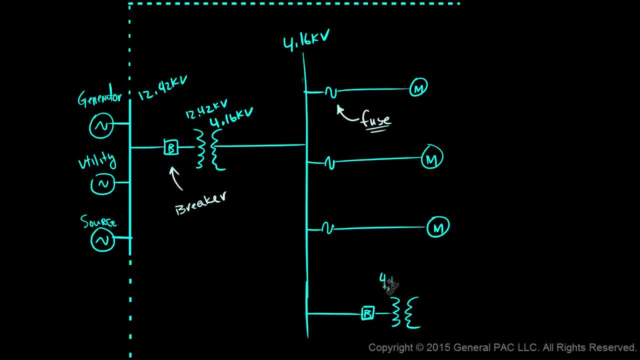 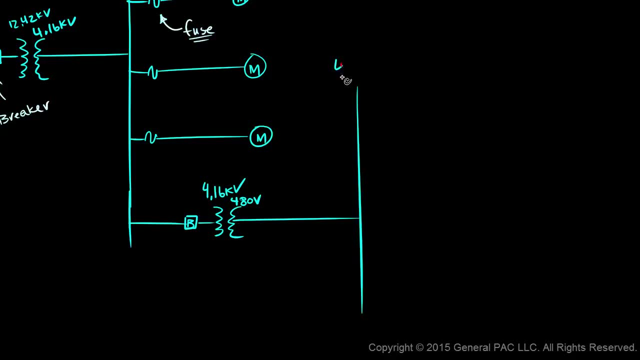 But that transformer steps that voltage down from 4.16 kV to 480 volts And we have another bus that's the 480 volt bus And taps off of the 480 volt bus which are fused. that's going to our auxiliary motors or our auxiliary equipment. 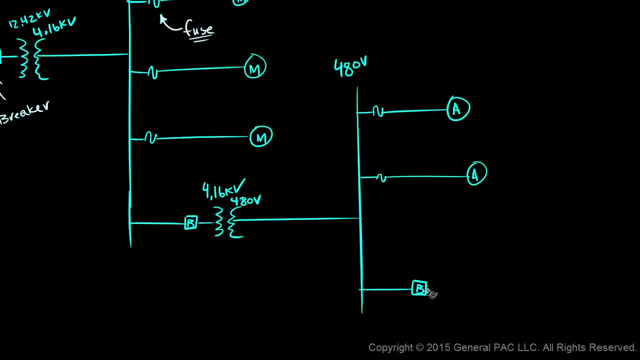 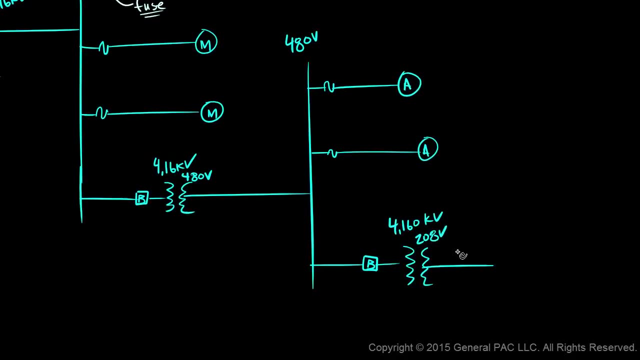 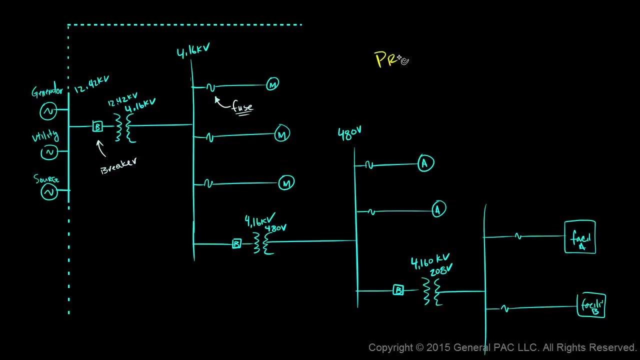 And then suppose we had another step-down transformer that was protected by a breaker that steps the voltage down from 4160 volts to 208 volts, And here we're feeding all the outlets of our facility. Okay, so a problem can be anything, right. 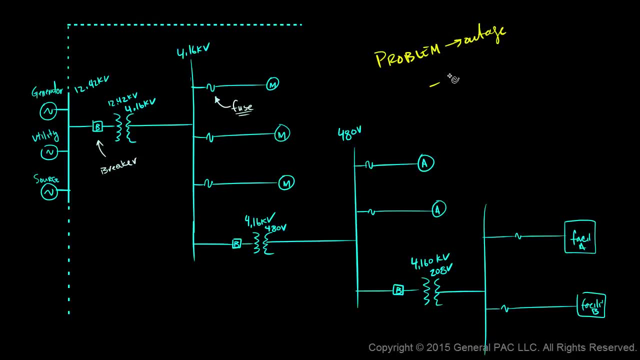 A problem that causes an outage. It could be various types of short circuits, It could be overloads, Harmonic problems, Insulation failure, Lightning, Loss of synchronism, Or simply human error Or natural disasters. So a problem is essentially an abnormality that's not normal or uncommon. 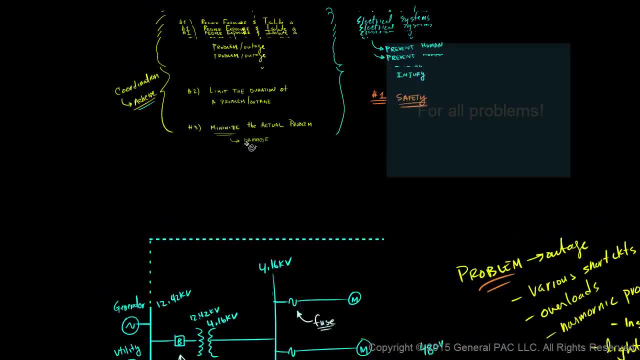 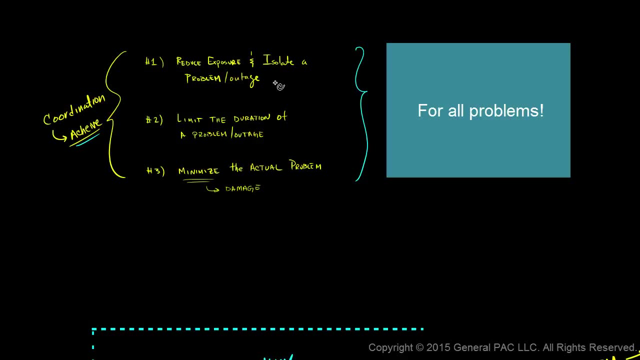 Okay, in our protection coordination it's supposed to do these three things: It's supposed to reduce the exposure and isolate the problem, It's supposed to limit the duration of the problem And it's supposed to actually minimize the actual problem. so the damage is minimal. 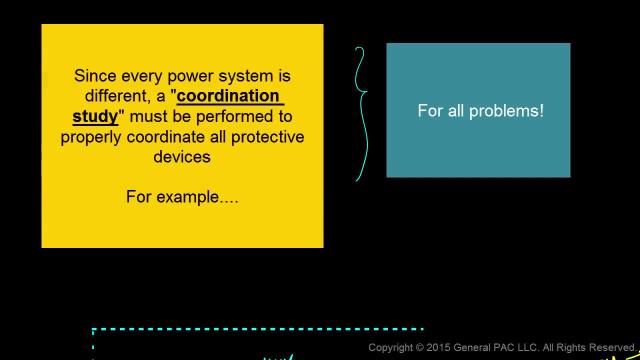 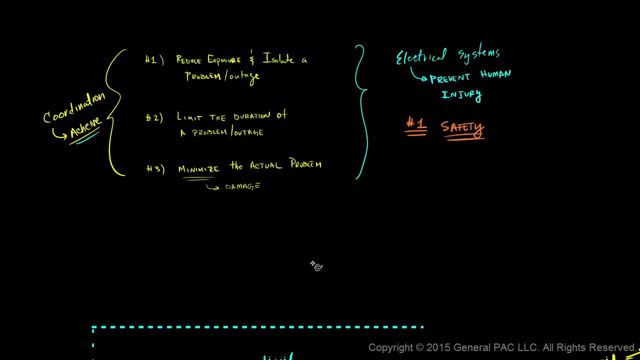 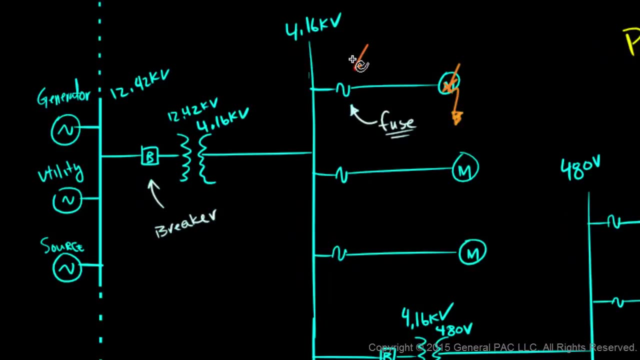 Okay, so let's see how that works. So suppose that we had a fault or any sort of problem on this motor. We should expect this fuse right here to number one. reduce the exposure of this problem, So reduce the problem area. 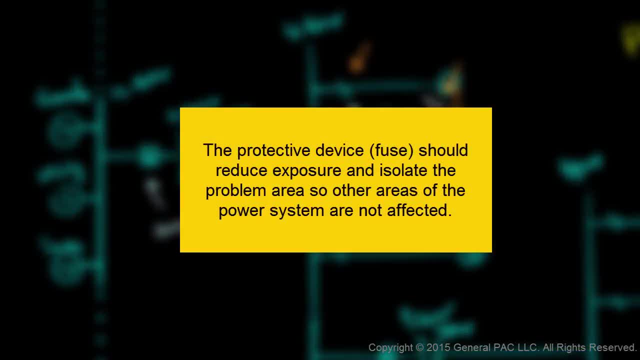 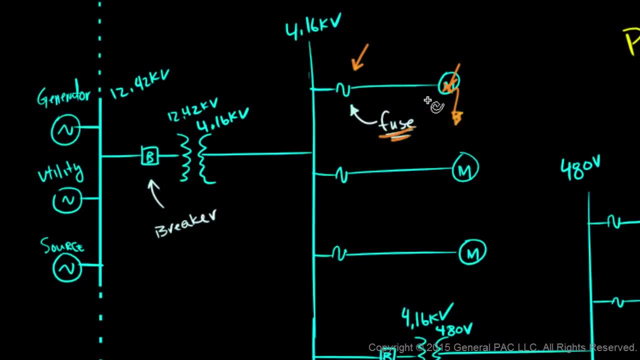 And it should also isolate the problem. Okay, it should limit the duration of the problem or the outage. And number three, it should minimize the problem. Okay, suppose that this fuse does not isolate the problem, So it does not isolate the problem. 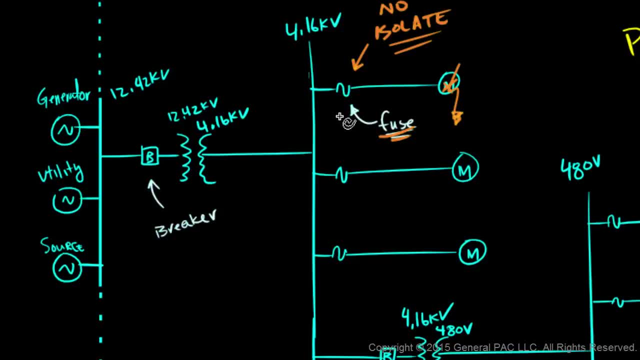 So, no, isolate this fuse. What's going to happen? Well, the next upstream device, which is this breaker. we should expect this breaker to isolate the problem. But what happens if this breaker isolates the problem? Well, what was a single problem on this single motor has now affected everything downstream.